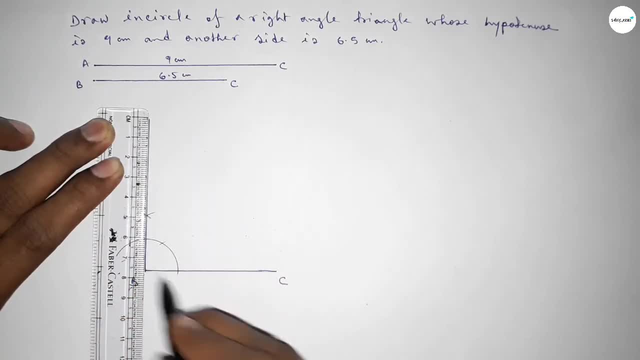 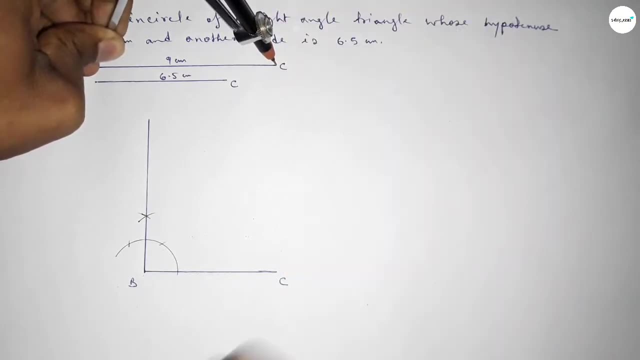 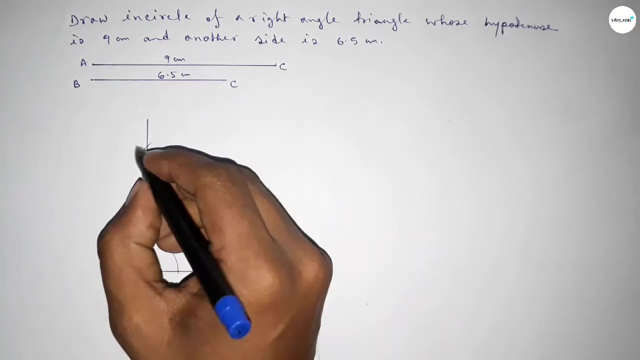 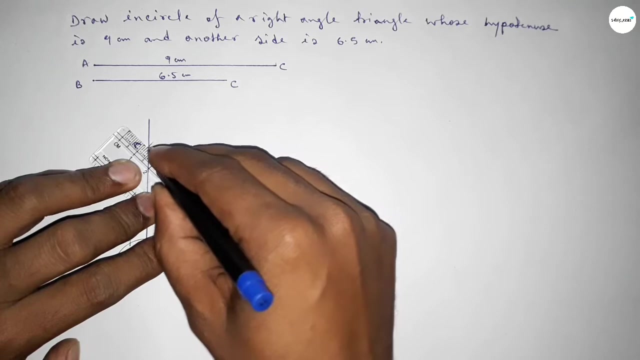 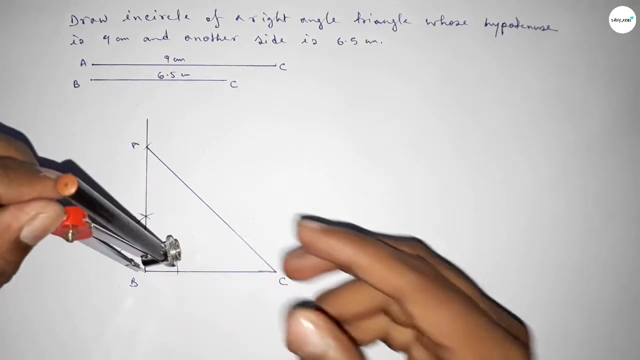 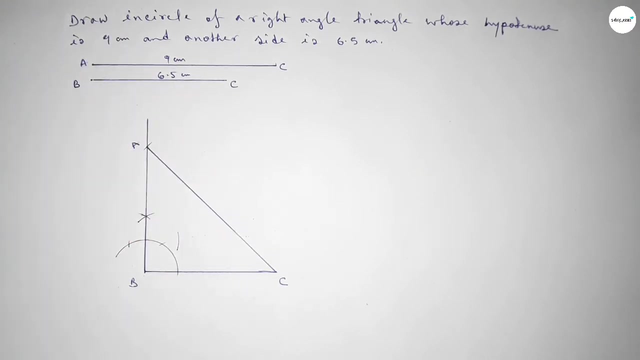 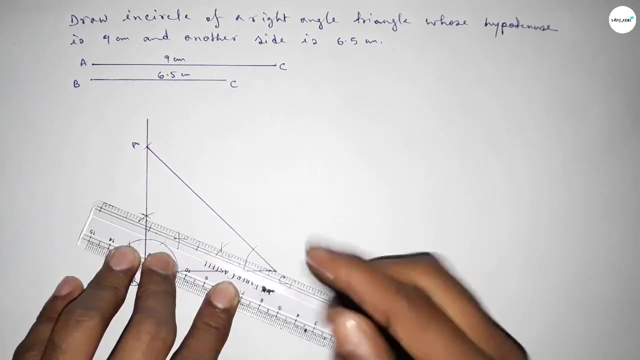 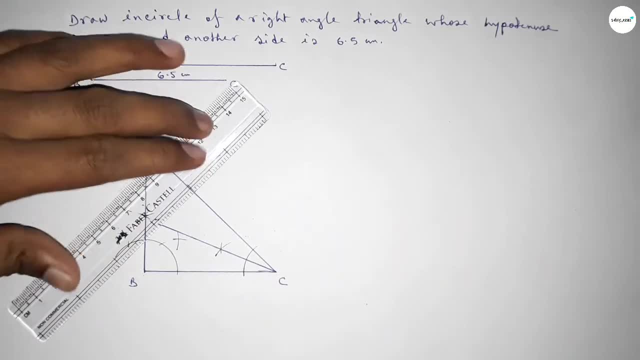 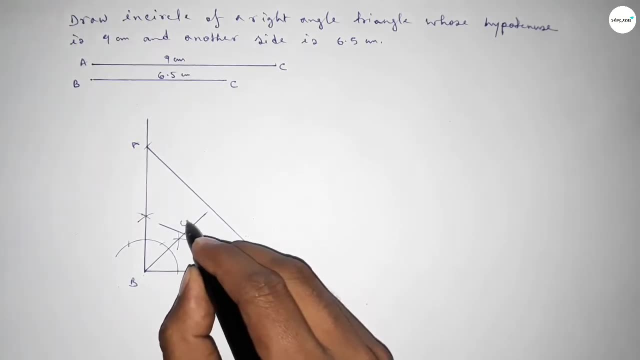 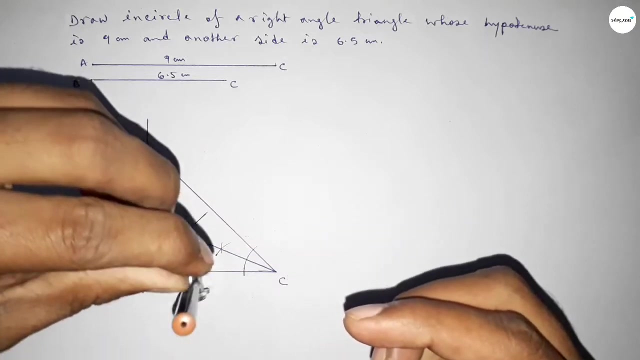 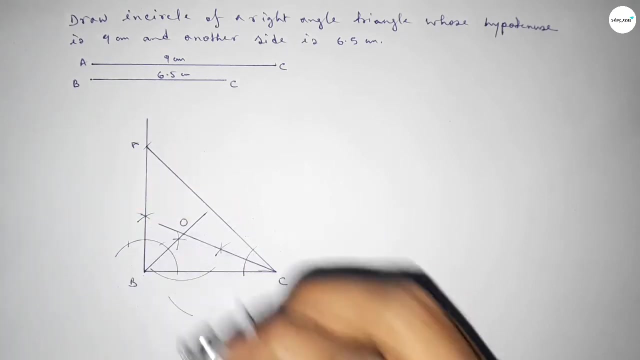 this and joining this bisector. both the bisector intersect at a point. this is taking o point. now we have to draw a perpendicular line from o to bc line. so taking any length and drawing a arc by this way, with same length, and putting the compass here and drawing a arc here with same. 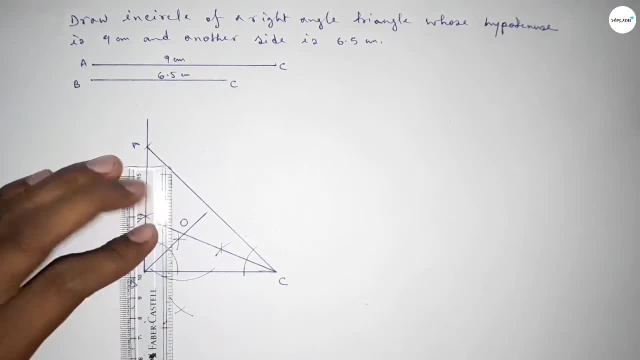 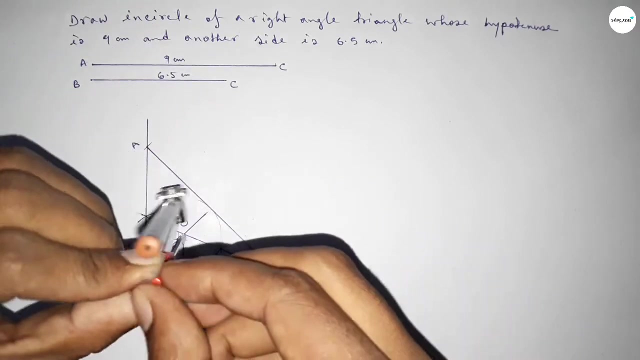 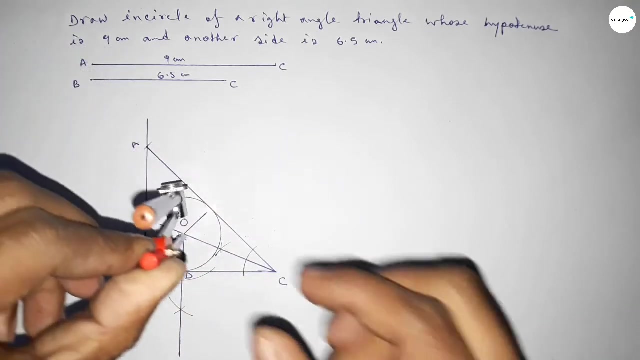 length and putting the compass here and cut here. now joining this to get the perpendicular line, so which intersect bc line at a point d, now taking the length od by using compass. next drawing a arc by this way and which represent a circle, and this is perfect picture. 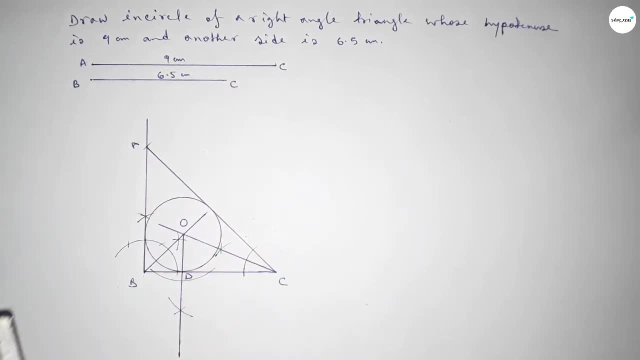 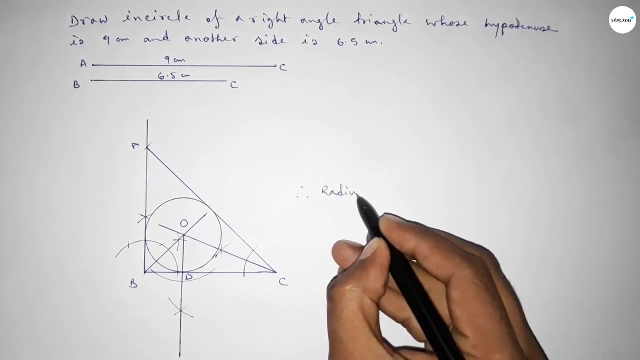 okay, now checking the radius, so this is 1.9. so radius od equal to 1.9 centimeter. that's all. thanks for watching. if this video is helpful, then please share.